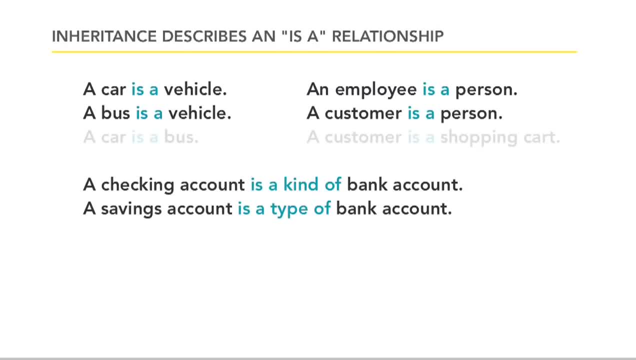 makes sense and what doesn't. We know that we can have multiple levels of this. A Bentley Continental is a car which is a vehicle. A Pomeranian is a dog, which is a mammal which is an animal. An inheritance is taking this idea, this form of abstraction that we do naturally in thought. 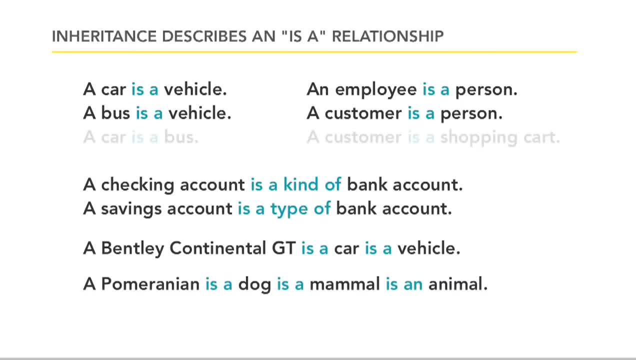 and language, and it's bringing it into programming. It's to allow us to identify that there might be shared attributes and behaviors between our objects And if we think about it, we can save some time and not reinvent the wheel. So here's where some people hit their first problem. They 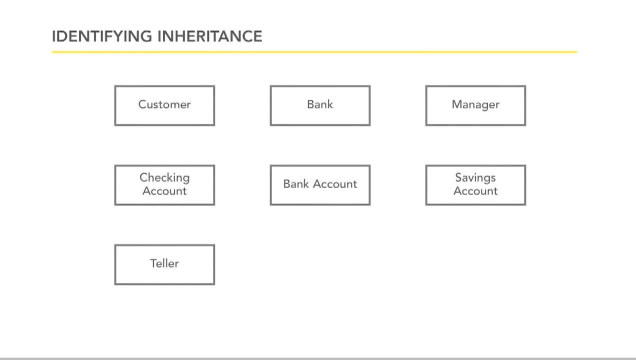 start sketching out a variety of classes, picking the nouns out of their written descriptions, And as we scan it we can tell there's some relationship between, say, bank and bank account. And we wonder, well, is that an inheritance relationship? And there's the question: Could? 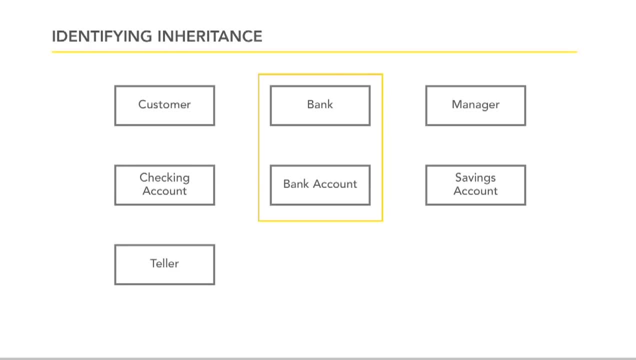 you say a bank account is a bank. Well, no, You wouldn't say that. Neither would I say a bank is a bank account. So there might be a relationship here, but it's not inheritance. But you could say: a checking account is a bank account or a. 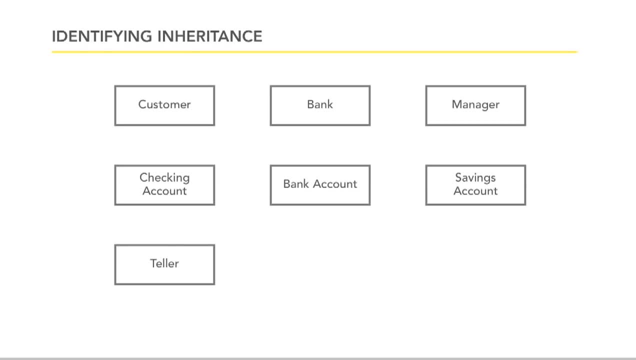 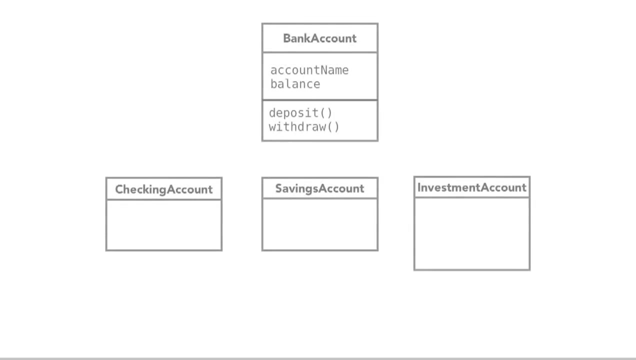 savings account is a bank account And it's a clue that we might be able to share some behavior in this area, But it's always. that is a question That should make sense when you talk about it in natural plain language. So the first class is shown with the open arrow. that looks like a wedge. One class points to the 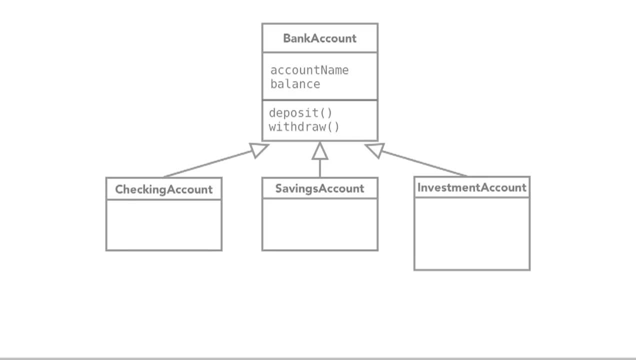 object it is inheriting from, otherwise called its superclass or parent class, And as soon as we say we're inheriting, we are considered the subclass or the child class And we automatically have all the attributes and behaviors from the class we're inheriting from. So in this case, bank account is 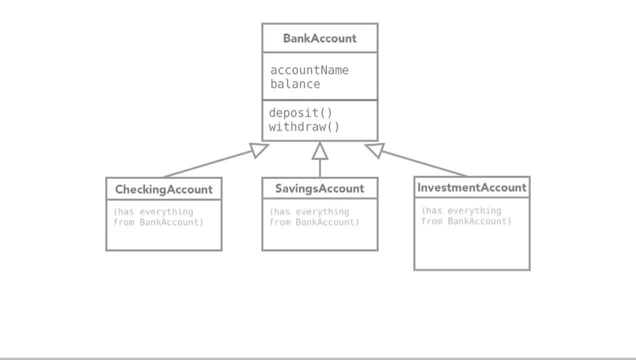 the parent class or the superclass Checking account, savings account, investment account. these are classes that would be considered subclasses or child classes. We bring in all the attributes and behaviors from the superclass, from the parent class, and then we can start adding some extra. 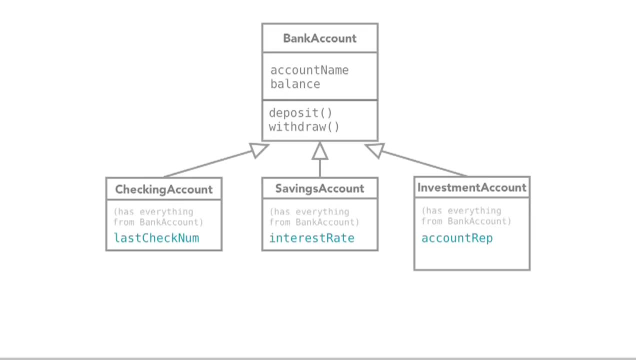 information. Sometimes we may want to change one of the behaviors we inherit from the superclass, And many languages allow a subclass to replace the implementation of a method defined in that super or parent class, And this is called overriding, And it lets us have more flexibility. 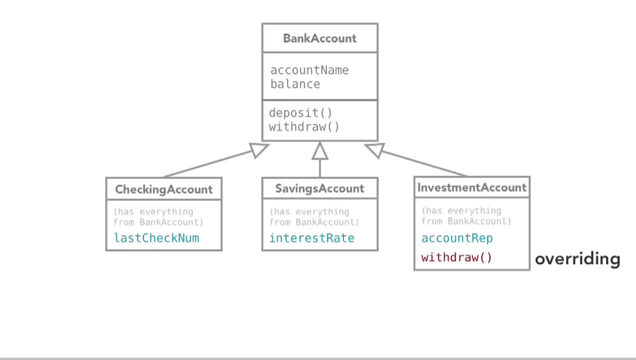 Most commonly it's not just to replace, but to do some behavior in addition to the inherited behavior. Now a word of warning: It is common for new object oriented developers to overemphasize inheritance and to come up with class diagrams with five levels for everything. Avoid this. Don't go looking for inheritance. 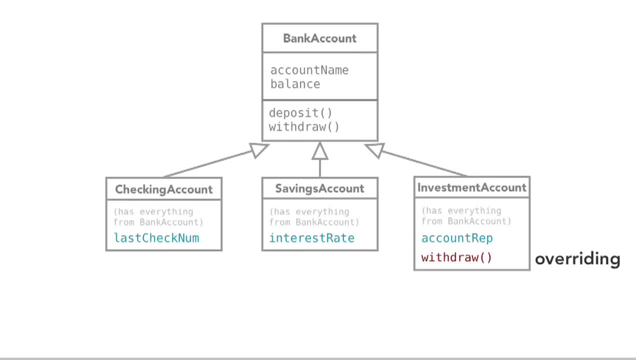 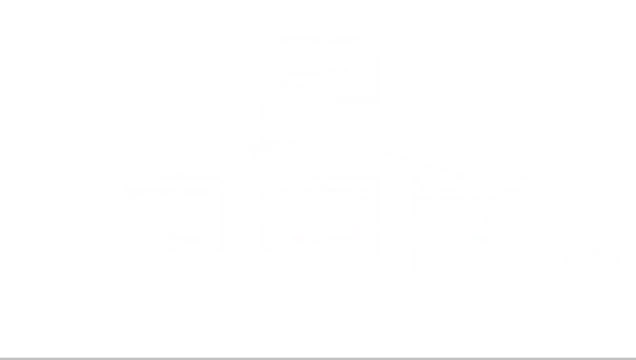 and don't stare at classes trying to figure out what their superclasses must be, because inheritance announces itself. You start building your classes for, say, a digital storefront and you start creating things like album and book and movie And you will notice if they start sharing a lot of common behaviors and attributes. 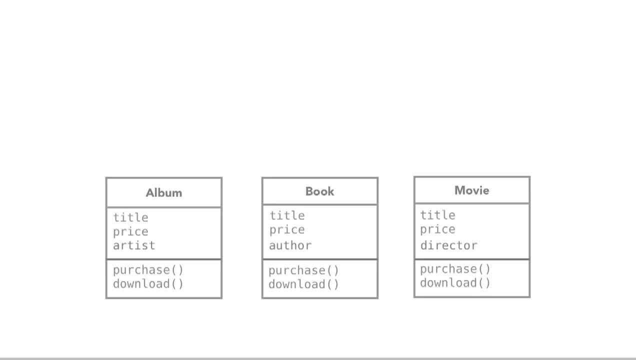 So in this case, we realize that we're sharing title and price as attributes and purchase and download as behaviors. So you may then create a superclass, trying to identify what's common between them all. Well, they're all products, And we'll create that. We'll strip out the similar behaviors and put them in that. 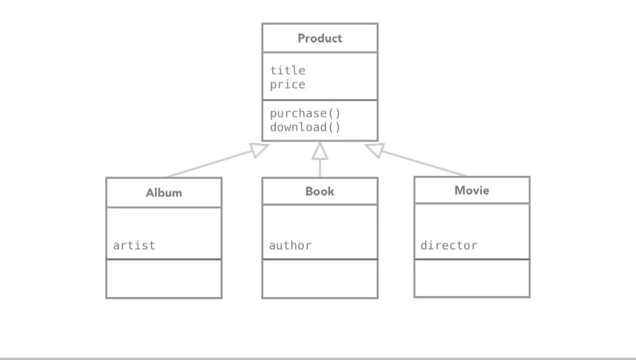 superclass In that parent class so we can identify and choose that commonality and then we will inherit from that class. But it should be obvious Now. sometimes it'll be identified from the bottom up, sometimes from the top down. You'll realize you have to create some more specialized classes, but let it occur naturally. 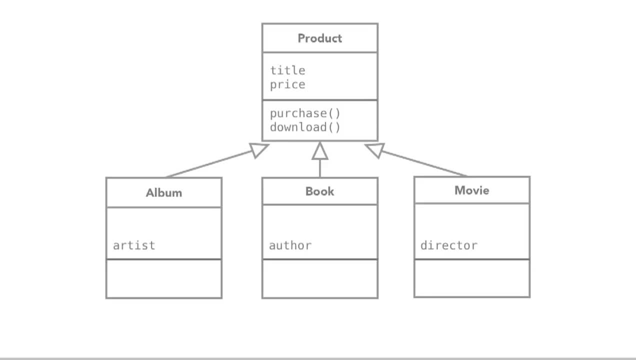 And if you create one or two class diagrams without any inheritance, that's not a problem. But do realize that inheritance is often vitally important in understanding existing object oriented programming environments, because the frameworks that you'll use in javanet, Objective-C, Ruby and others 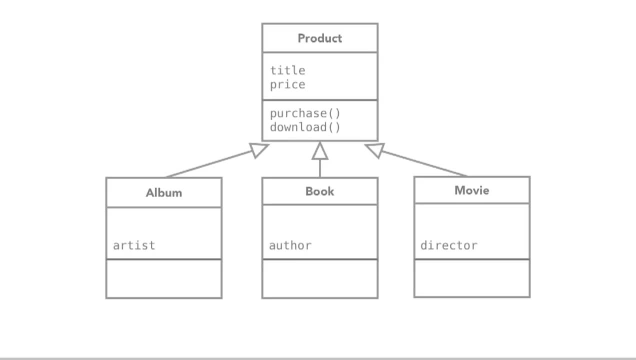 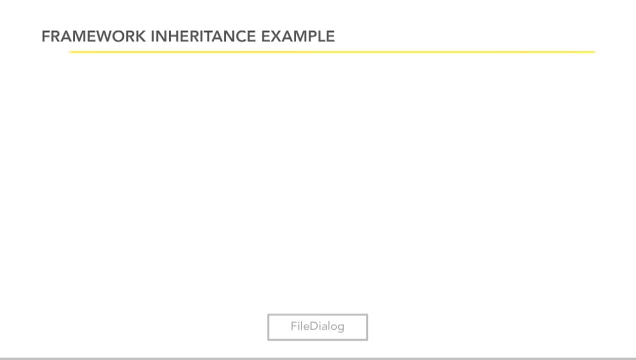 often use inheritance substantially because they're trying to provide generic and extensible frameworks rather than writing a specific application. In Java, for example, there is a built-in file dialog class which we can use Well. it inherits from a dialog class which inherits from the window class.